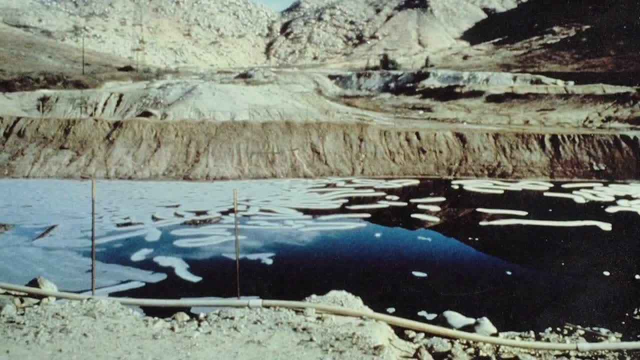 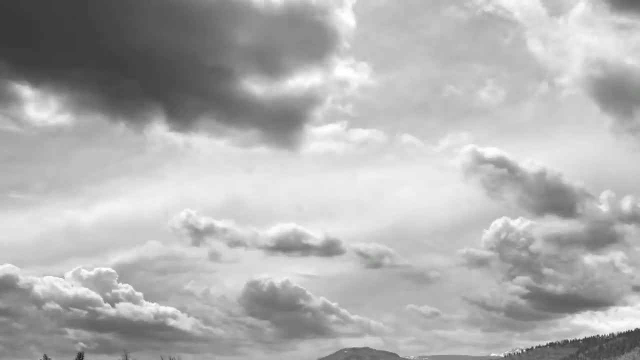 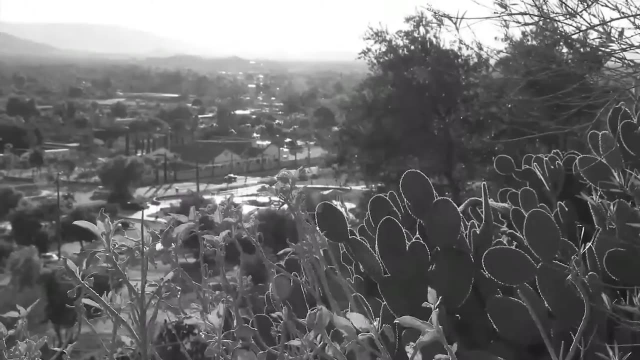 More than 32 million gallons of liquid industrial waste were disposed in unlined ponds, including acids, caustics, metals, solvents and pesticide byproducts. When the site would overflow, liquid contamination would flow into the community, Eventually exposing children at an elementary school to a variety of toxic chemicals. 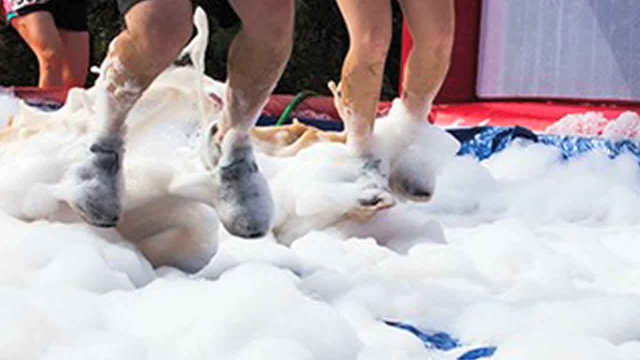 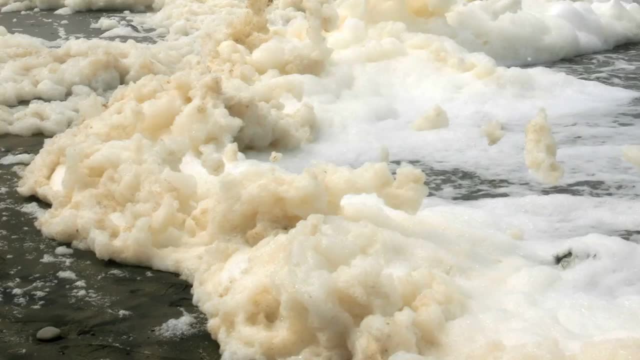 These were very dangerous chemicals. My two boys, being little boys, were playing in the puddles and splashing around. We had kids there making beards out of the foam And the youngest one, who was the one who played in the puddles and was into everything. 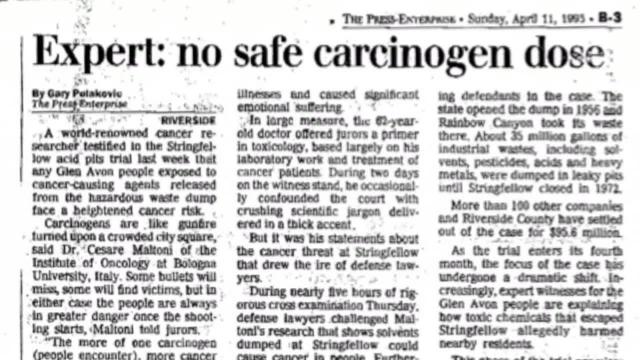 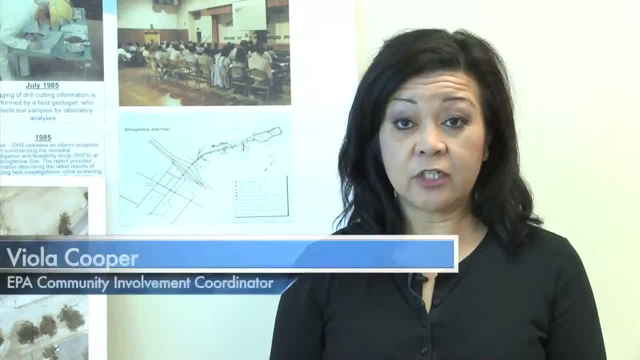 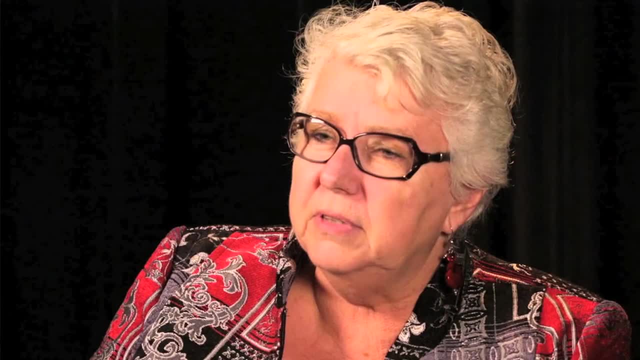 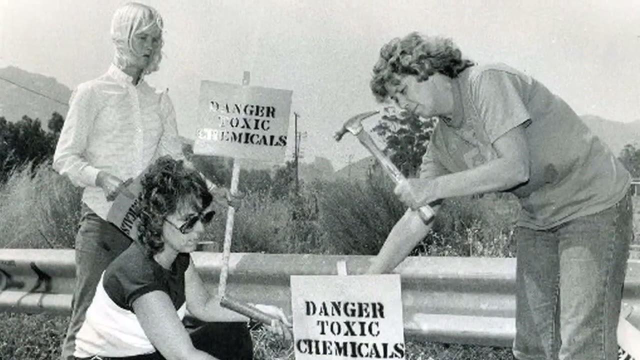 would come home from school talking about being dizzy and having blurred vision And he started experiencing seizures. The community started organizing and having community meetings and this is where we saw Penny move forward and just be that community leader. It changed my life. We need to not just sit back and elect people or let agencies do things. 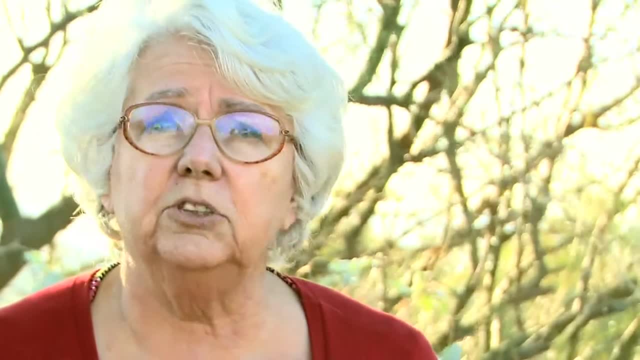 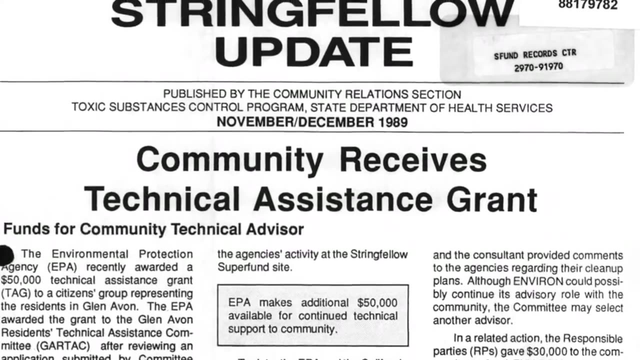 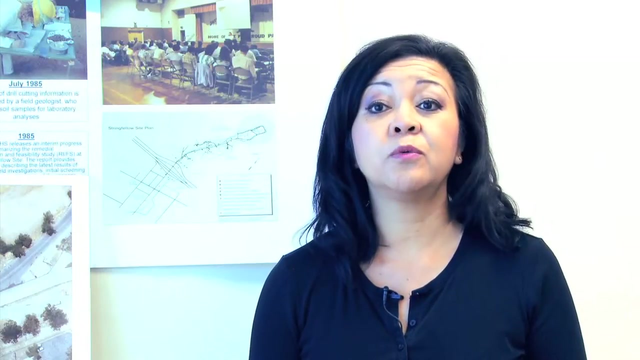 We have a responsibility to make sure that things are done correctly. Out of Penny's hard work we modeled the Technical Assistance Grants Program, the TAG program. If it wasn't for Penny rising up at that moment, we wouldn't be where we are today. 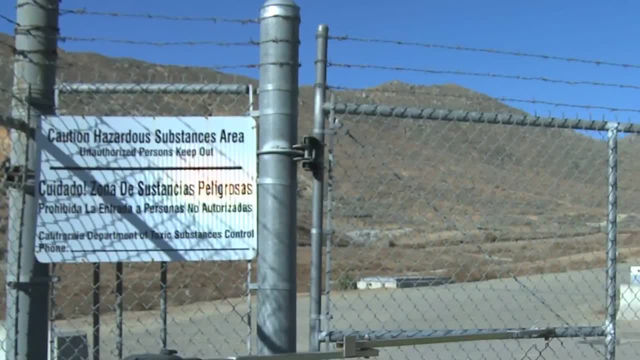 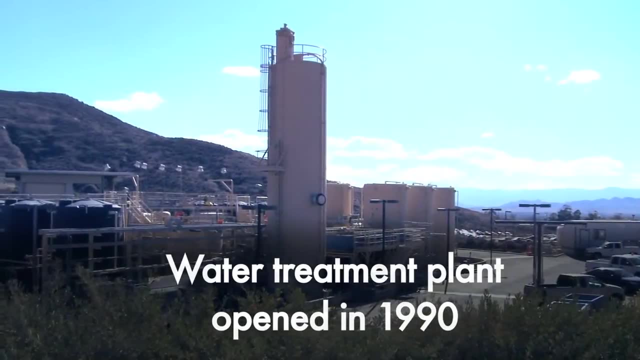 To prevent any chance of future spills into Pirate Creek, the remaining liquid waste were pumped from the disposal ponds. in the late 70s, Contaminated soil was excavated and a groundwater extraction and treatment system was installed in the canyon to prevent contaminated groundwater from reaching the community south of the site. 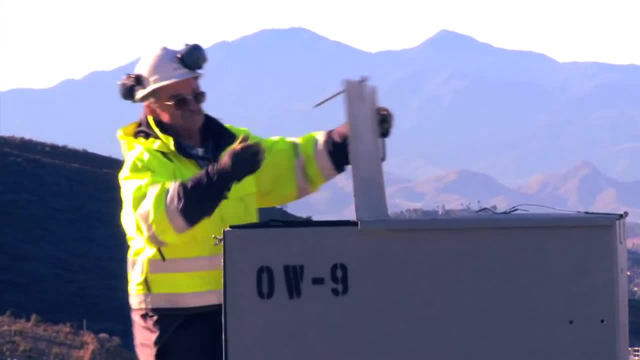 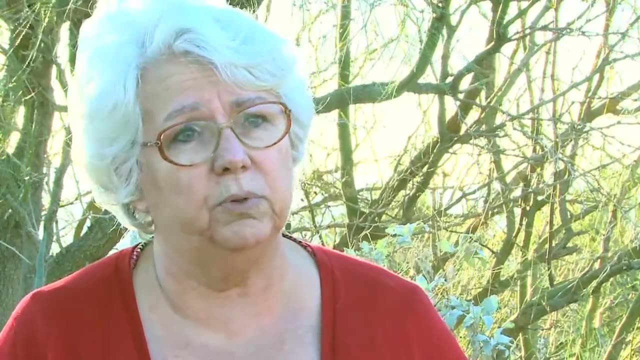 While there is more work to do, EPA is proud of the progress that has been made with our state partners And that the current remedy is protected. Thank you, The staff that is there. I have great respect for them. I think that's the most important part is for us to listen and then get that feedback. 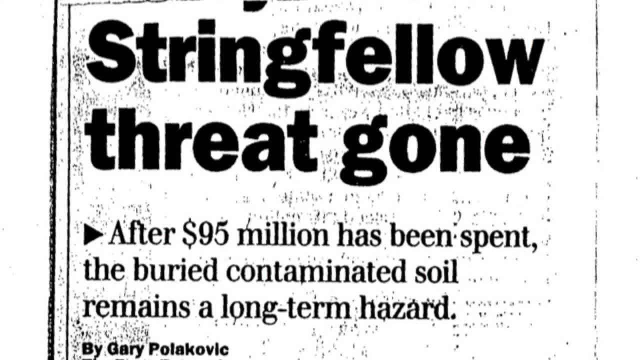 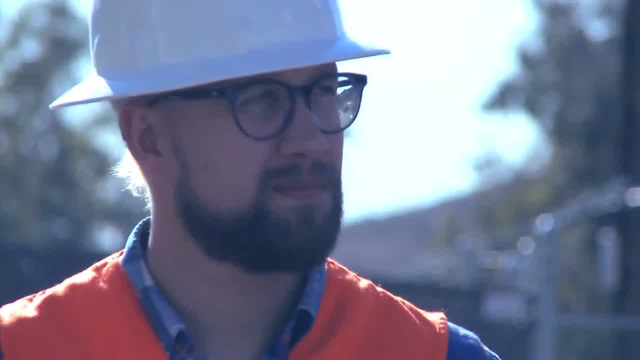 And that's that feedback and that input process that Superfund is all about. You know, our democracy really works and it only works if people are involved. Looking back on 35 years of Superfund, we've made a great deal of progress in Stringfellow. 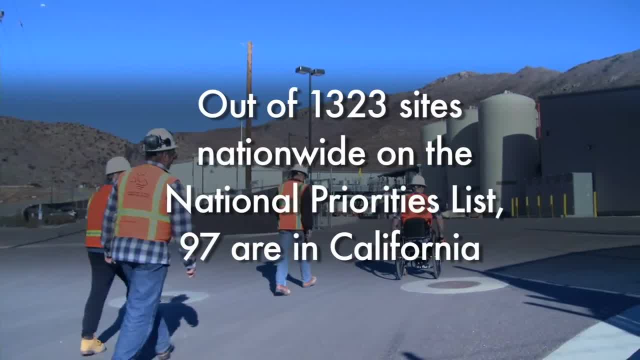 and at other Superfund sites, to continuing the great work with our communities to protect human health and the environment.